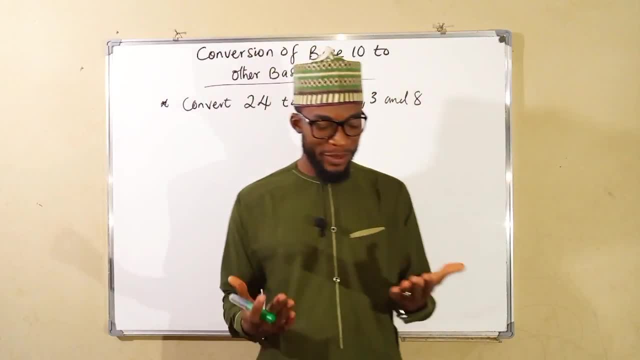 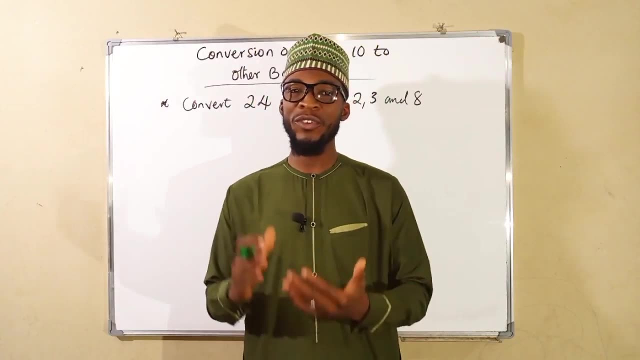 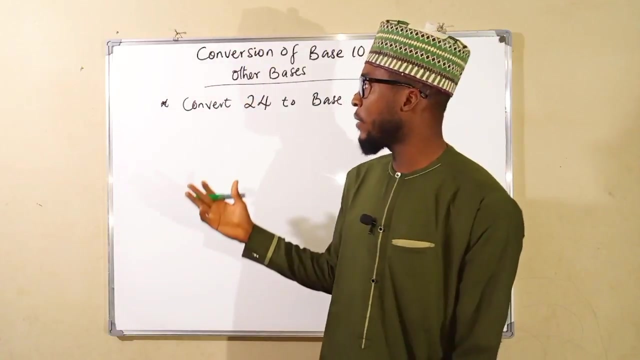 Hello, good morning viewers. In our previous lesson we have seen the introduction of number based system and I promise our next class is going to be a conversion of base 10 numbers to other bases and other bases back to base 10.. So this is the question I have. We are asked to convert 24 to base 2, 3 and 8.. Let us 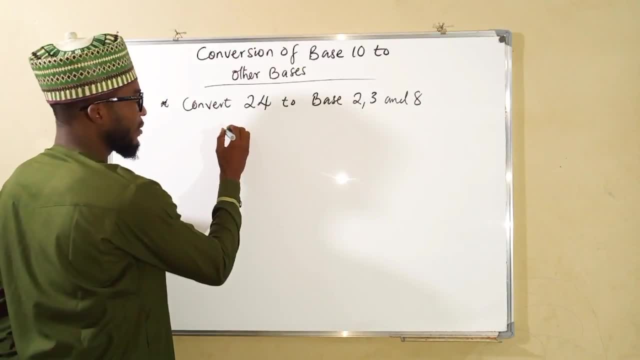 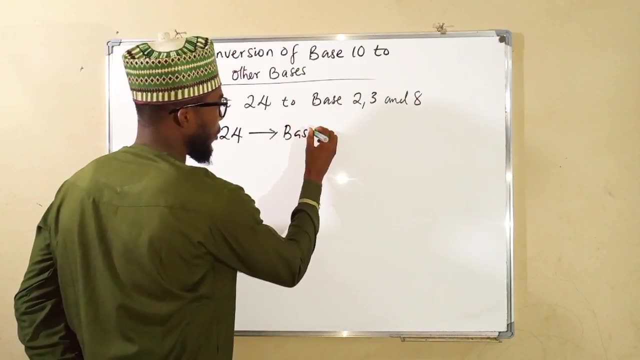 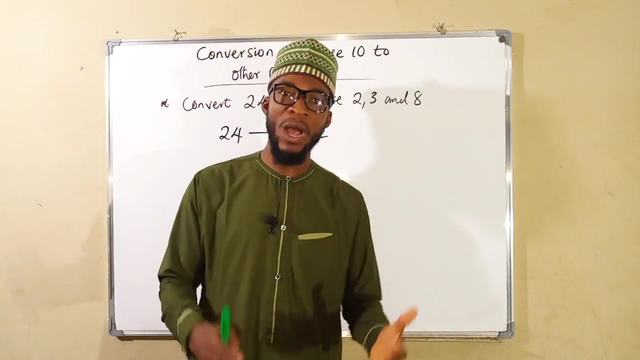 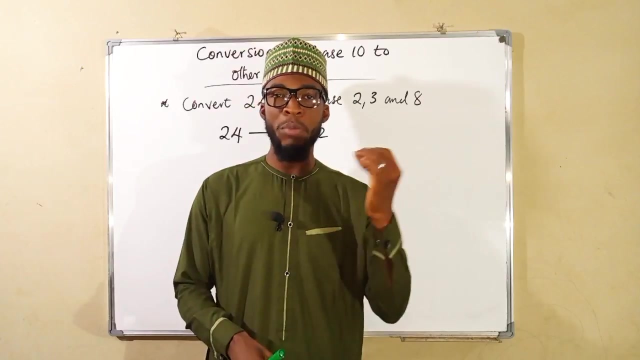 start with base 2.. We want to convert 24 to base 2.. In number based system, numbers in base 10 are sometimes referred to as the binary numbers or the decimal numbers, while numbers in base 2 are referred to as the binary numbers. Now, 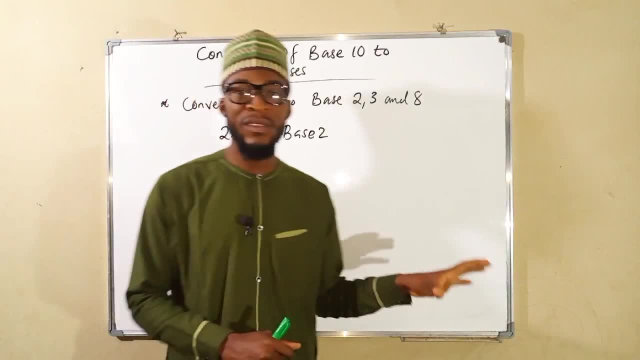 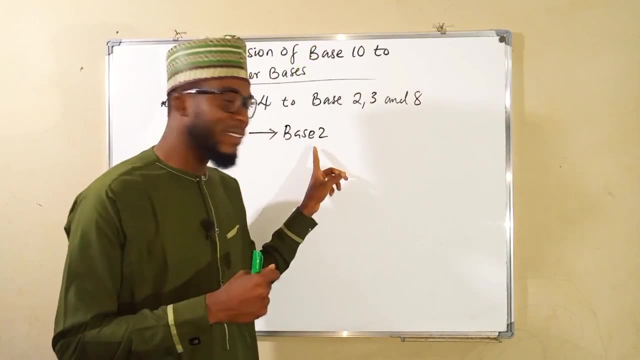 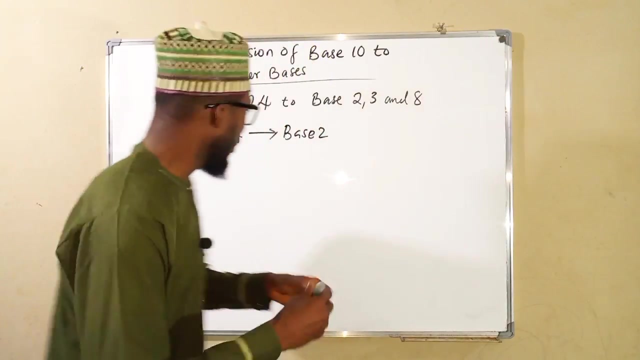 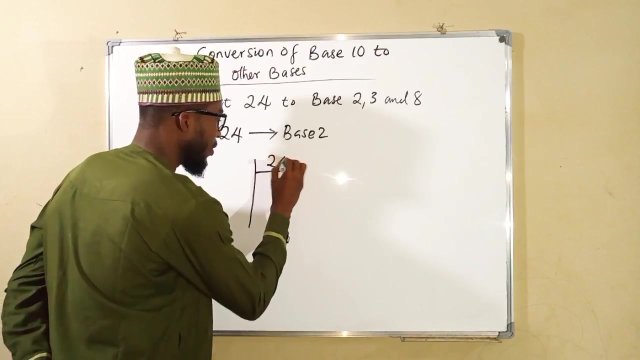 to convert numbers from base 10 to other bases, you need to perform a successive division of that number in base 10, using the assigned base, and collect the set of the remainders in their descending order. Let us divide this 24, and you remember 24 has no base, so I told you any number. 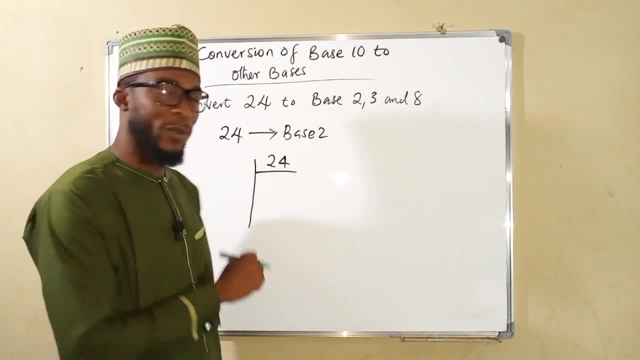 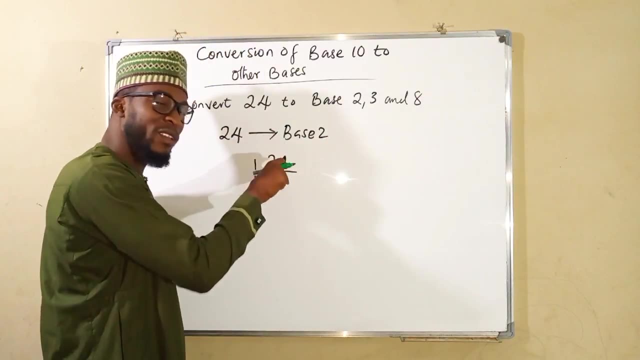 without an assigned base is base 10.. So this 24 is in base 10.. So this 24 is in base 10.. So this 24 is in base 10.. We want to convert it to base 2.. Therefore, we are going to divide this 24. 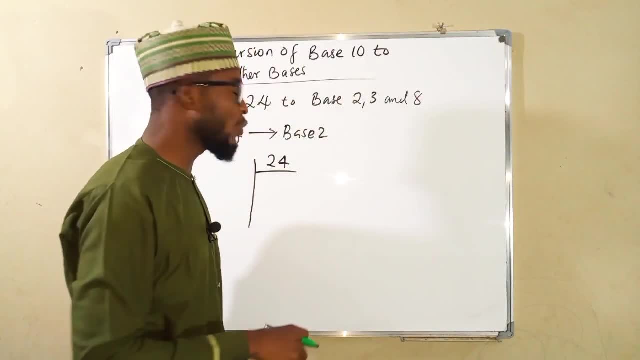 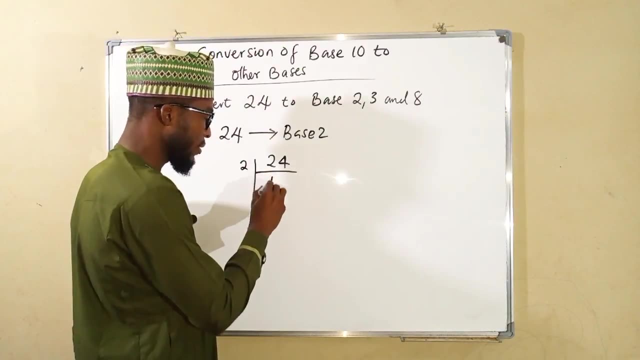 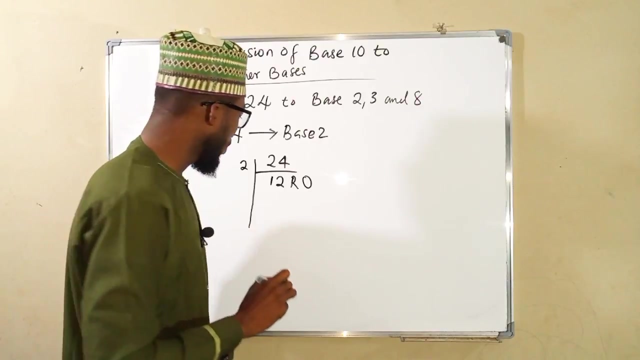 continuously till we reach the last number which 2 cannot divide. So we have 2 here. 2 can go into 24, 12 times without remainder. Therefore you write: remainder 0. You continue. 2 can go into 12, six times without remainder. 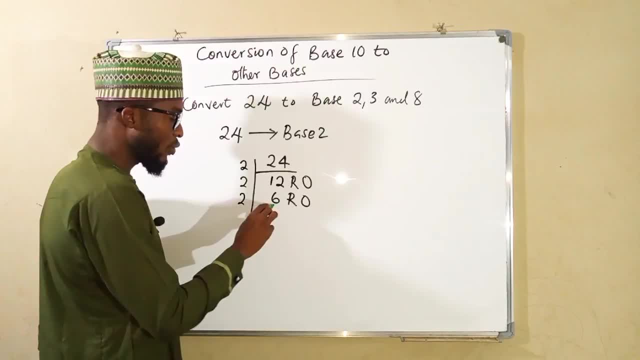 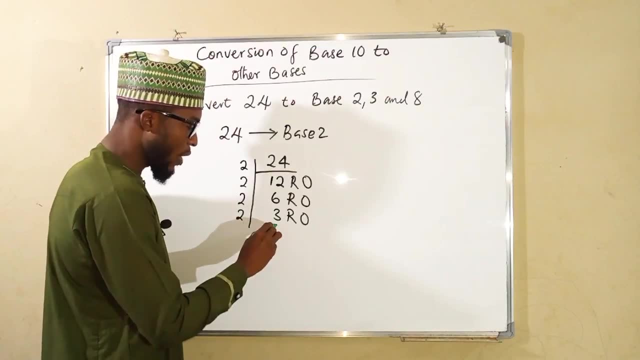 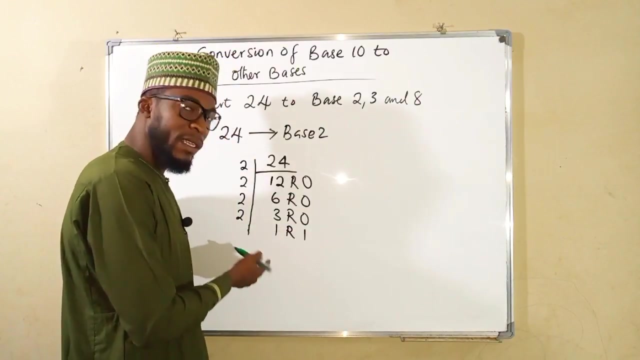 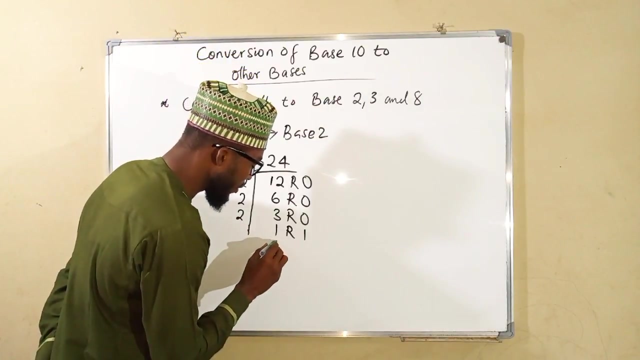 so there is no remainder. Two as well can go into six three times without remainder. Two can go into three one time, but we have one left remainder one and lastly, we know two cannot go into one. therefore we stop, Then we collect the set of these numbers in this form and we 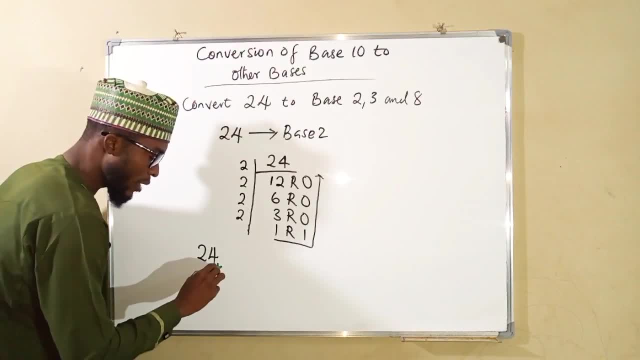 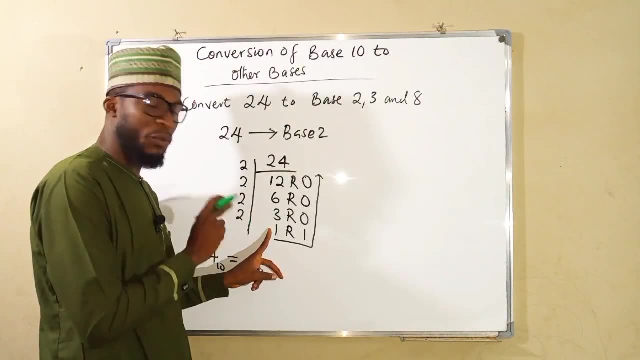 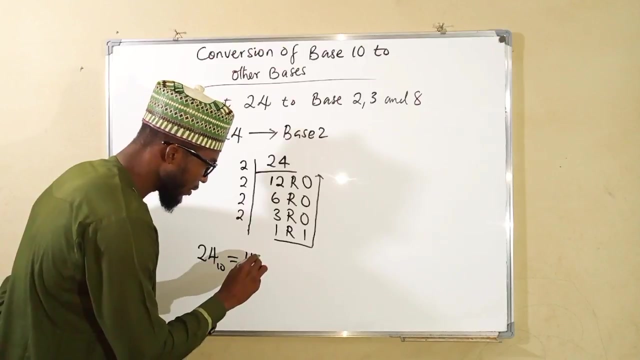 conclude by saying: 24, which is a number in base 10, is equal to. you start from this number. whatever number it is, you start with it. we have 1 1 0 0 0. we have 1 1 0 0 0, but this number is in base 2. 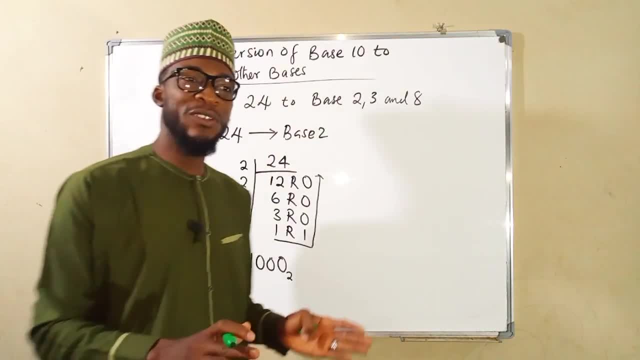 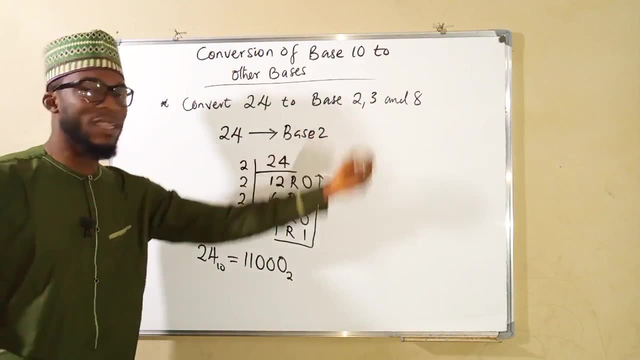 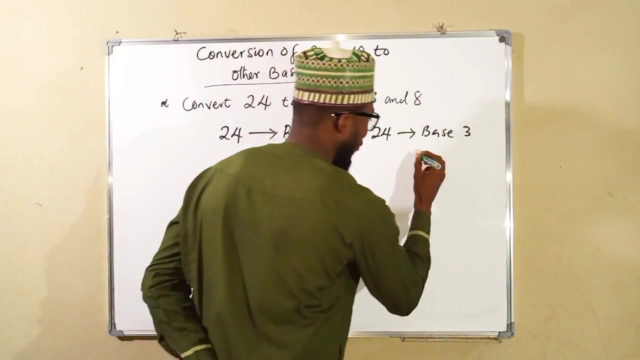 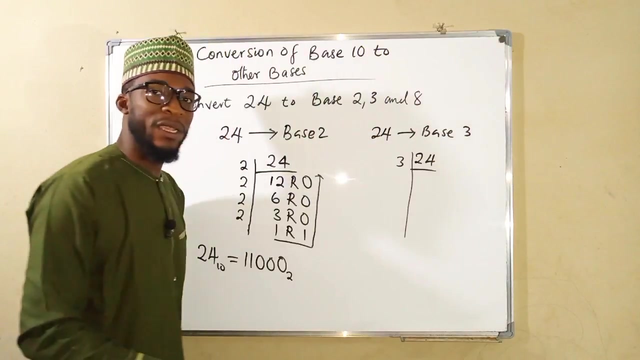 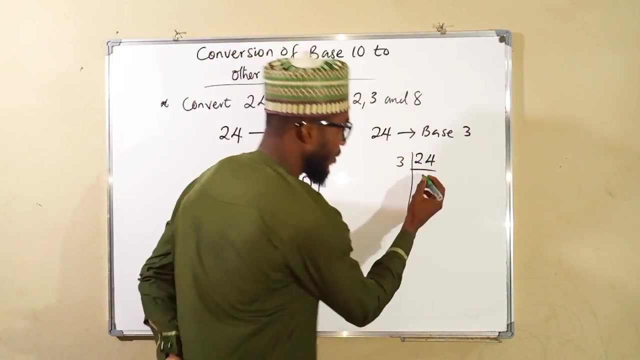 hence this number and this number are exactly the same, just that they are in different bases. Now let us see the conversion of this number to base 3.. We write 24 here, which is a number in base 10.. We divide 2 by 3. Three can go into 24 eight times, without remainder. 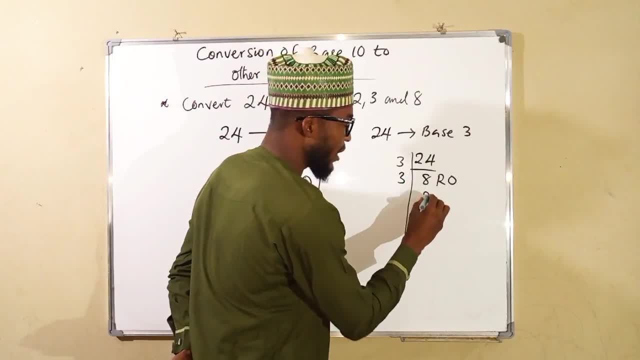 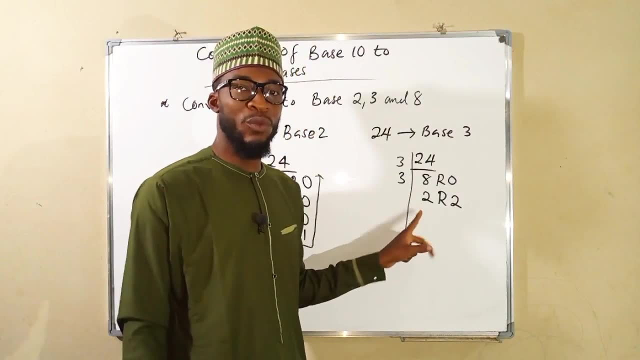 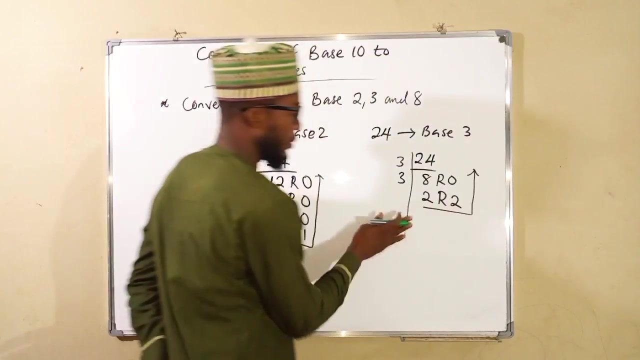 Three can go into two is equal to eight, two times which remainder of two. But three cannot go into two. therefore, you stop and take these numbers in their descending order. Therefore, 24, which is a number in base, 10, is equal to. you start with this one. 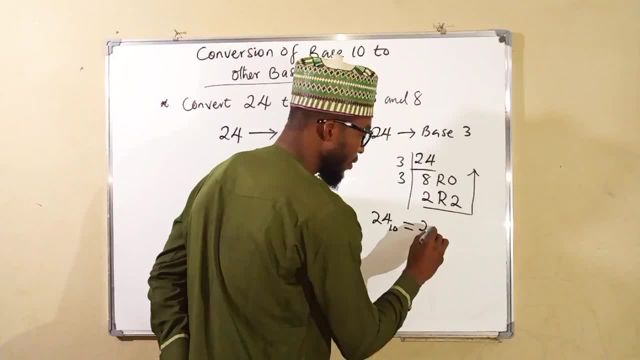 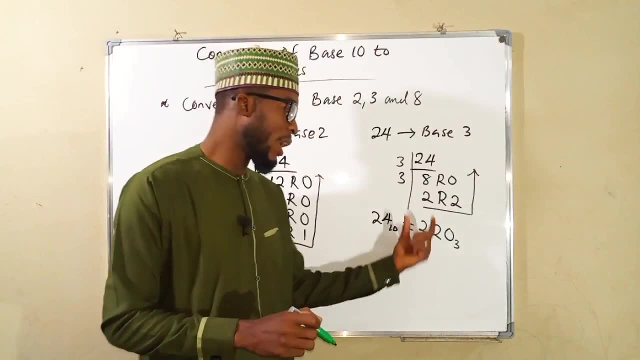 2, then followed by this 2 and lastly we have 0, but this is two, and the previous first two lines have six is in base 3, and hence 24 and 2, 2, 0 are exactly the same, just that this one is in base 10, while 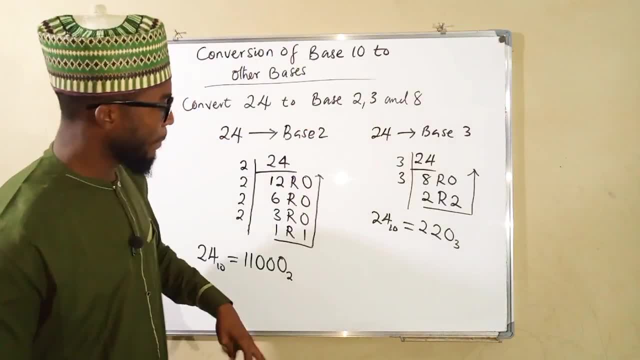 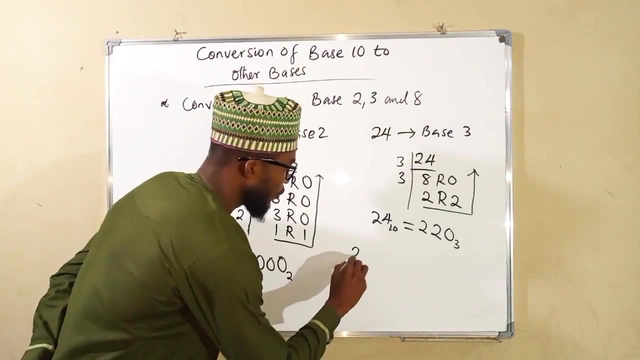 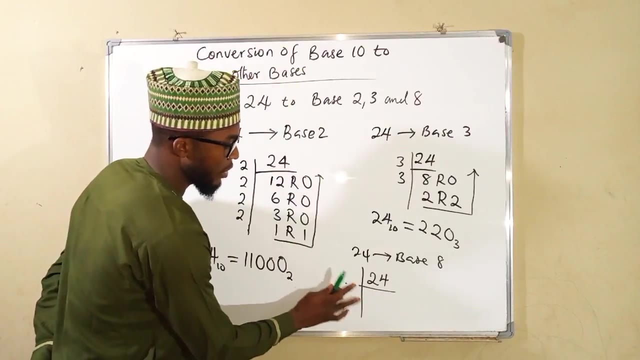 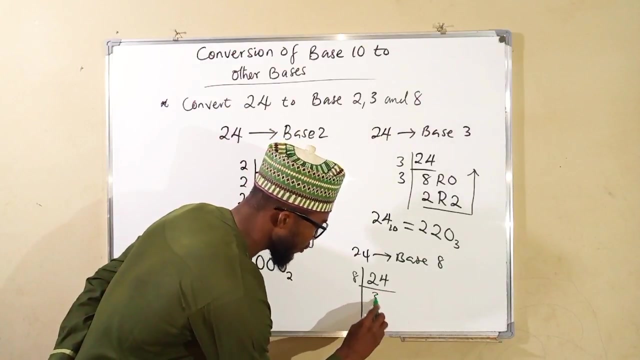 this one is in base 3.. now, lastly, let us see the conversion of this number 24 to base 8. we have our 24. we divide through. i know 8 can go into 24 three times, so we have 3, without reminder. 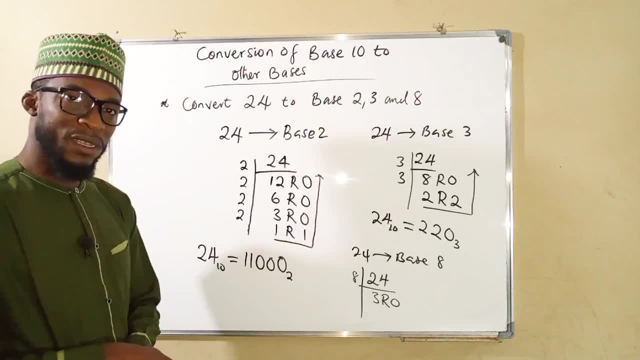 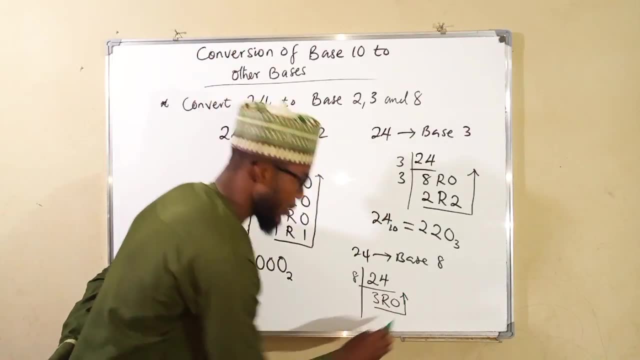 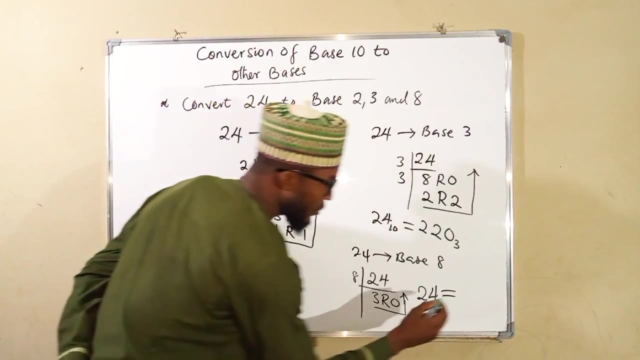 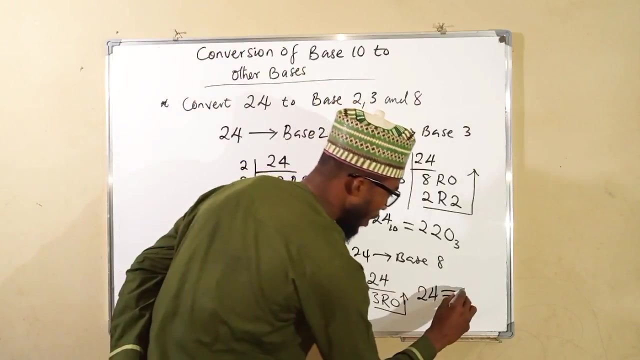 and 8 cannot go into 3, and hence you stop and take your values in their descending order and conclude by saying 24 is equal to: we have 3 and 0, because you always start with the number here, then you go here and upward, so we have 3 and 0, but in